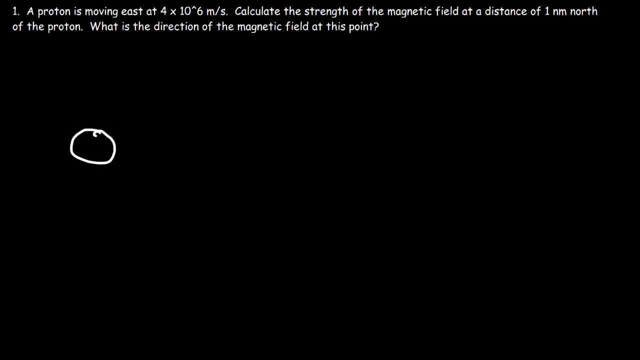 start with a picture. So the direction of the velocity is to the right and we want to calculate the strength of the magnetic field at a distance of 1 nanometer north of the proton, So let's say at 0.8.. How can we do that? The 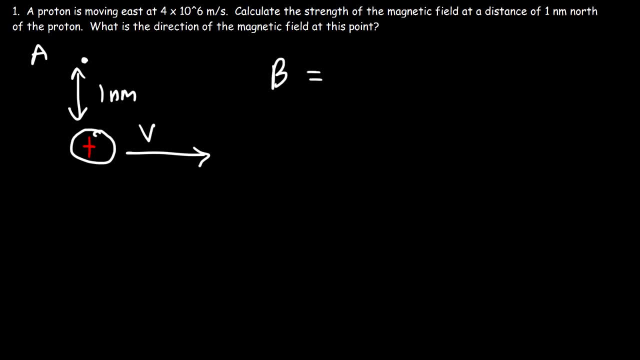 formula that you need is this: equation B: the magnetic field is equal to the permeability of free space divided by 4 pi times Q. this is going to be the absolute value of Q times the velocity multiplied by sine divided by R squared. Now let's go ahead and plug everything in, So the 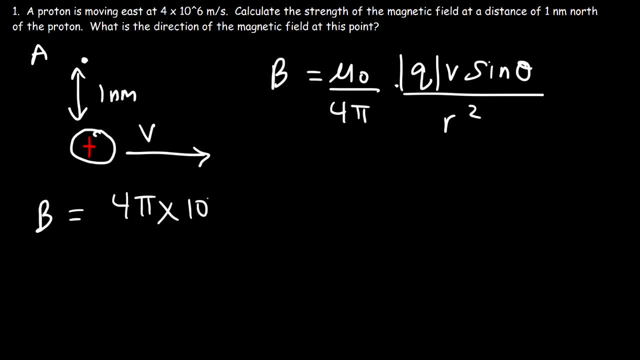 permeability of free space is 4 pi times 10 to the minus 7 and the charge of a proton is 1.6 times 10 to the negative 19 coulombs. And we don't need an absolute value for this case. it's already positive. Now the speed is 4 times 10 to. 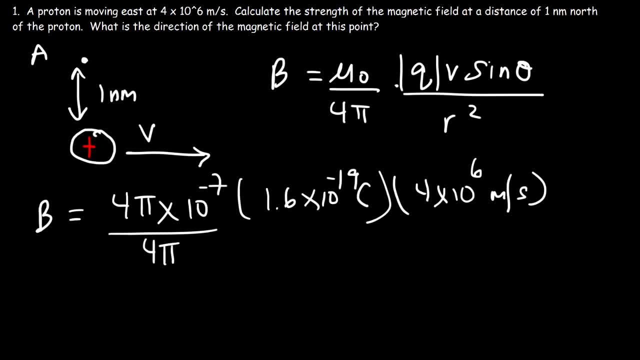 the 6 meters per second. And then the angle, So V is in the positive x direction. R, if you go from the source point, which is the positive charge, to the field point, which is where we wish to calculate the magnetic field, R goes from source to field. so R is basically this vector and 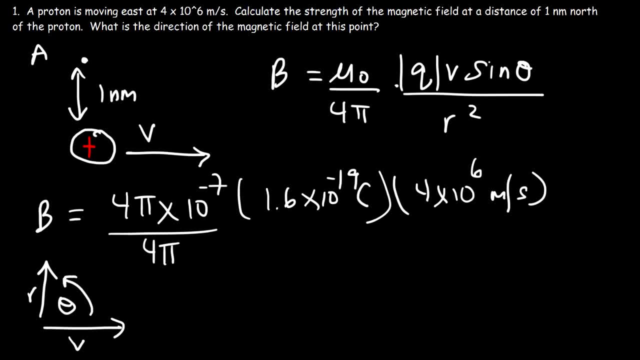 this is the angle between them, So because they're both perpendicular to each other, the angle is 90.. and R is 1 nanometer, which is 1 times 10, to the negative 9 meters, and let's square that. 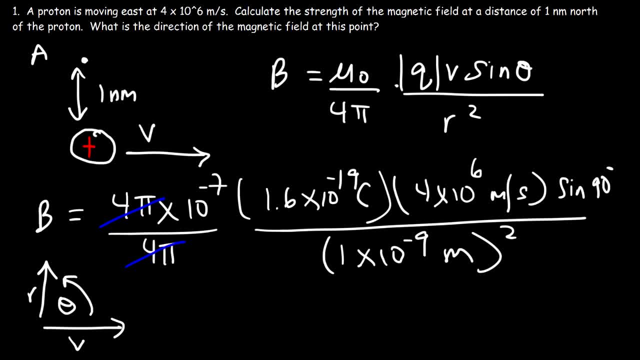 Now 4 pi divided by 4 pi, these two can cancel. so that's 1 times 10 to the negative 7, multiplied by 1.6, times 10 to the negative, 19, times 4 times 10 to the 6,. 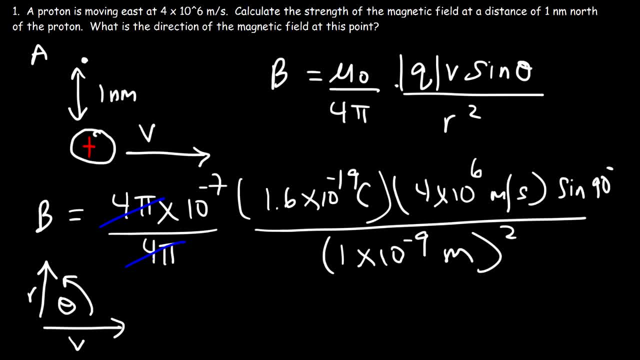 sine 90 is 1, so we don't have to worry about that, and divided by 1 times 10 to the negative 9 squared, So the magnetic field at 1 nanometer from the proton is 0.064 tesla. 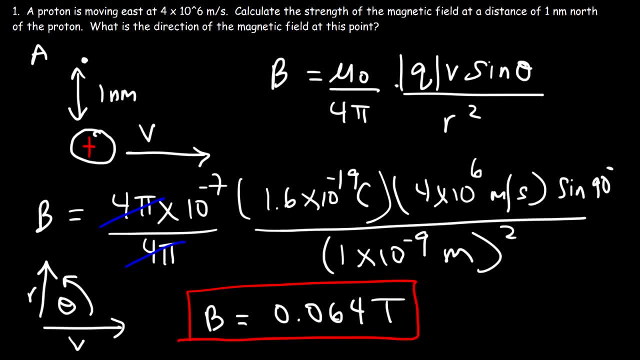 So, as you can see, the strength of the magnetic field increases greatly as you get close to a charged particle. It's inversely related to R squared. So what happens to the strength of the magnetic field if you double the distance? 1 over 2 squared is 1. fourth, 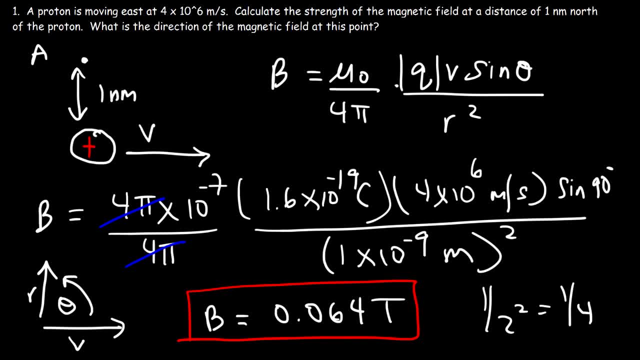 So if you double the distance between R squared and R squared point A and the charged Q or the proton, the magnetic field will decrease by a factor of 4.. Now, if you triple the distance, the magnetic field will decrease by a factor of 9.. 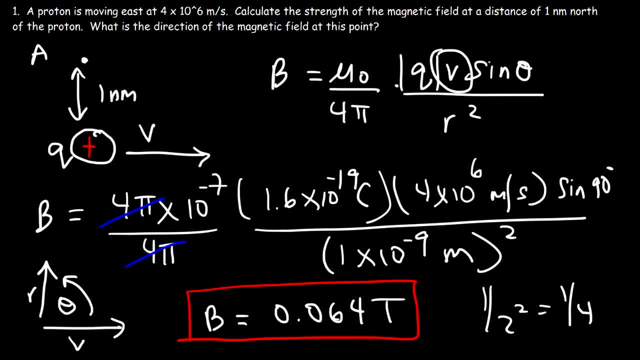 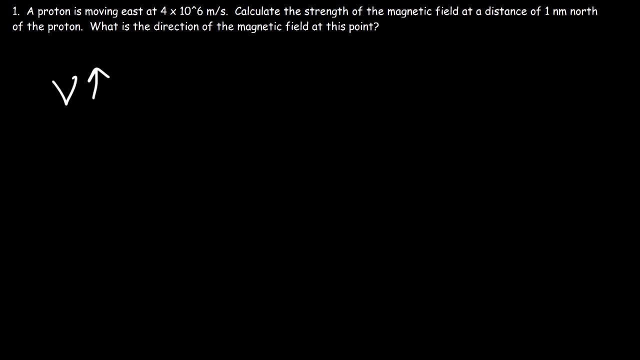 1 over 3, squared is 9.. If you double the speed of the proton, the magnetic field will double in value. If you triple the speed, the magnetic field will triple. See, You need to know this. As the speed of the particle increases, the strength of the magnetic field increases. 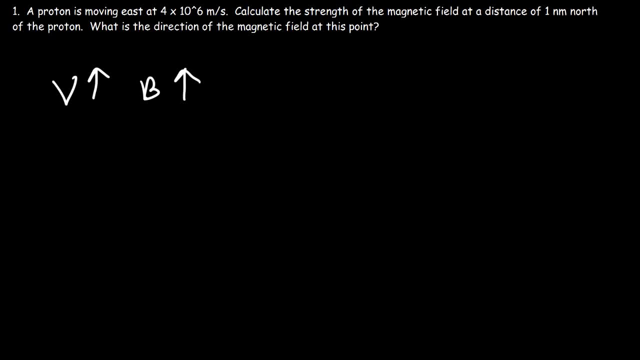 So only moving charged particles can generate a magnetic field. A stationary charged particle will not generate a magnetic field. If you increase the distance between the charge and the point in which you wish to determine the magnetic field, that magnetic field will decrease as you move away from the moving charge. 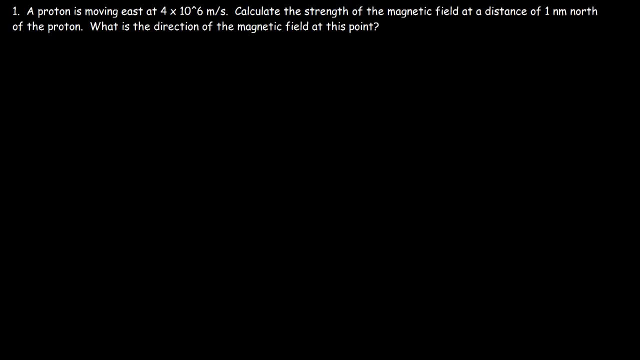 So now, how can we determine the magnetic field, How can we determine the direction of the magnetic field at that point? So how can we do that? Well, we could use the right-hand rule, And so this is the velocity. 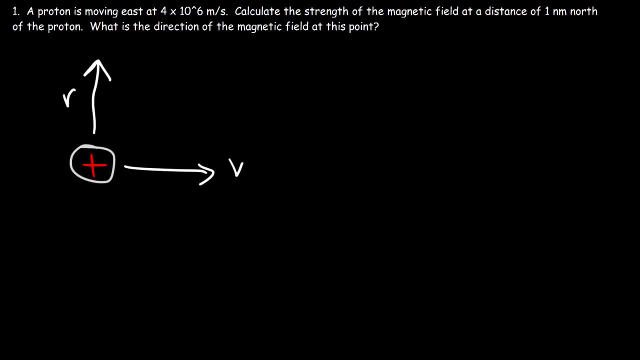 This is the position vector. And where is the magnetic field? So here's another formula that you can use: B is equal to mu zero over 4 pi times Q Times the cross product of those two divided by R squared Now, R hat is also the position vector divided by R. 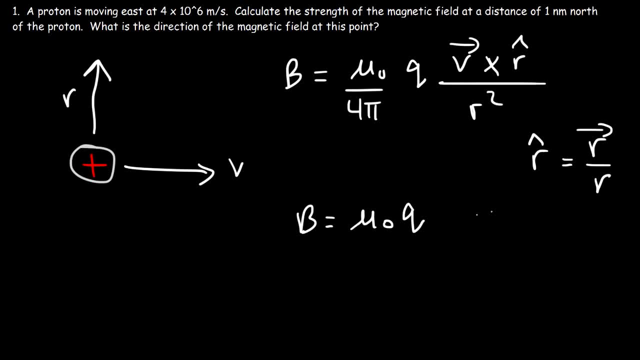 So you can also write the equation like this, if you want. So this would be 4 pi R cubed If you use the position vector in that way. Now we're going to focus on this term right here: The cross product of the velocity vector and the position vector. 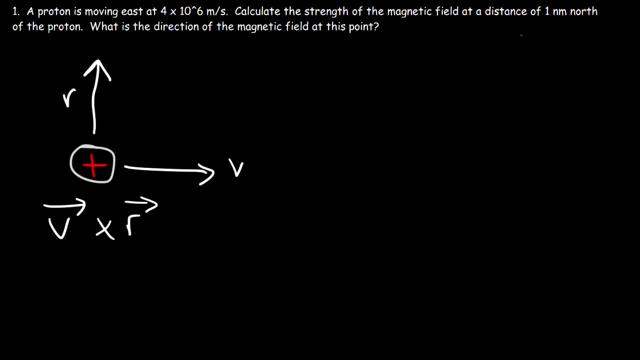 And that's going to help us to determine the direction of the magnetic field. So, using the right-hand rule, this is going to be first, because it's on the left side, This is going to be second And this is going to be third. 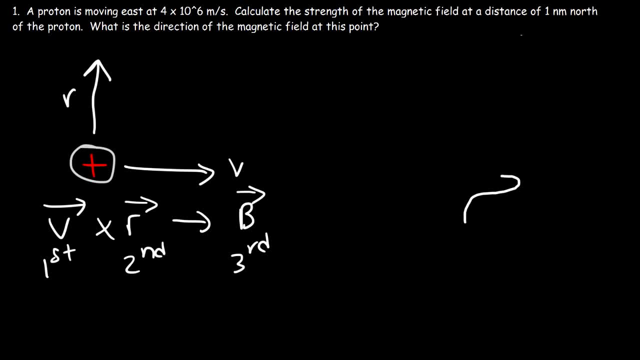 So first point your thumb in the direction of the first vector on the left, which is the velocity, And then your four fingers point it in the direction of the second vector, which is the position vector. So V is directed east or in the positive X direction. 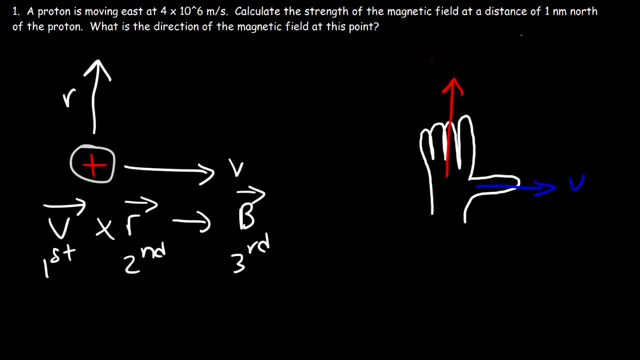 And R is directed north in the positive Y direction. The magnetic field, the third vector, should be coming out of the palm of your hand. So, basically, if you align your hand based on what you see on the page, it should be coming out from where your hand opens up. 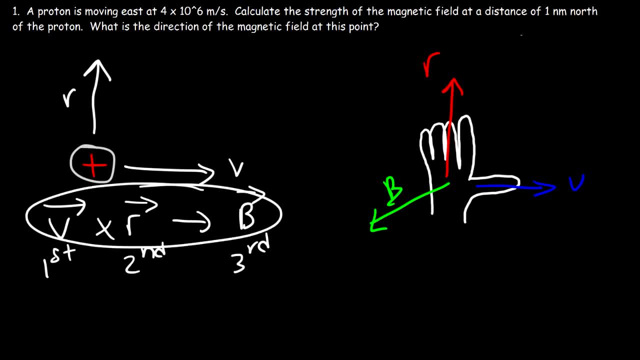 So make sure you understand this When you wish to find a cross product of two vectors in order to get the direction. the first vector, the one that you see on the left, that's going to be associated with your thumb. The second vector is associated with your four fingers. 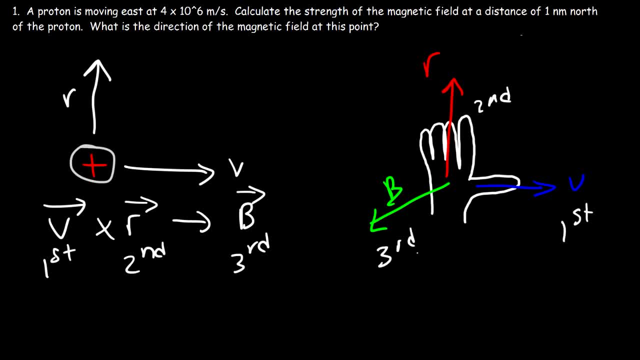 And the third vector comes out of the left, And the third vector is the one that you see on the right out of the palm of your hand. Now, in some other videos, I've shown another technique in which you can get the same answer. if you don't like the right hand rule, I call it. 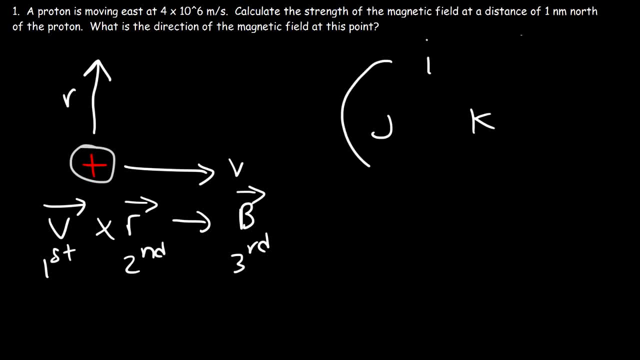 the IJK technique. So if you're traveling counterclockwise it's positive, And if you're going clockwise you're going to get a negative answer. So just keep that in mind. So we need to find the value of V, cross R, at least the direction, and that's going to give us the 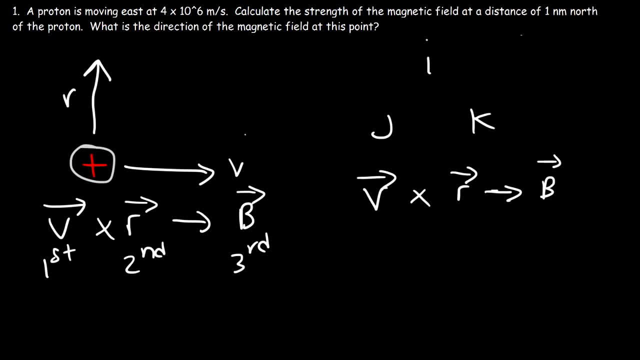 direction of the magnetic field. So the velocity is in a positive X direction, which is associated with I, and the position vector is in a positive Y direction, which is associated with positive J. So we need to find a cross product of I and J. So start with the first vector, I. 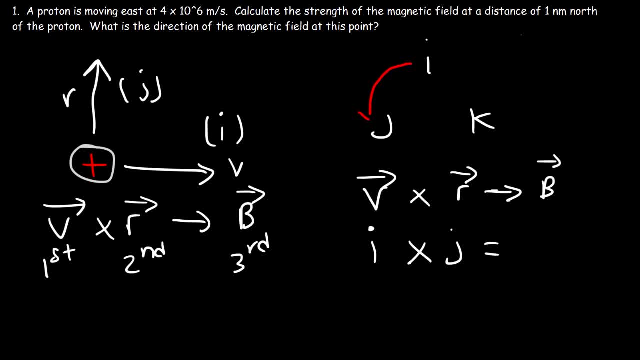 which is in the I direction, I mean, and go towards the second one, which is towards J, and then that's going to equal K. Now, since we're rotating counterclockwise, we're going to get a positive answer, because it's either two answers that it can be. 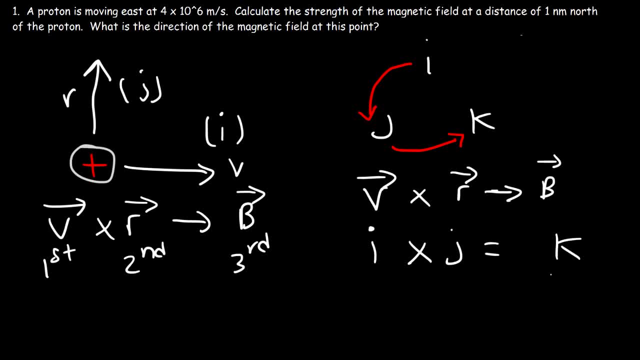 positive K or negative K. So because we're rotating counterclockwise, this is going to be positive K And this answer is in agreement with what we had. We said the magnetic field was coming out of the page, So we're going to use a circle to represent that, If it's coming out of the page. 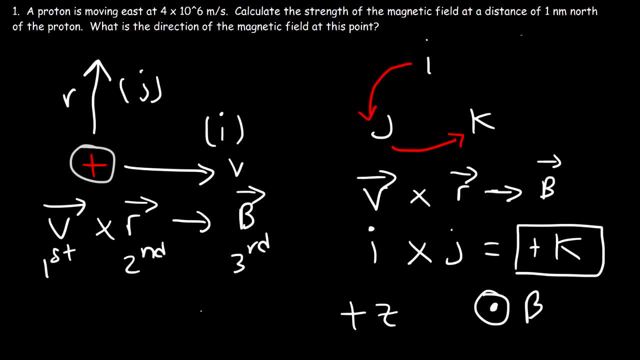 that means it's going to be positive K, So we're going to use a circle to represent that. If it's coming out of the page, that means it's coming in a positive Z direction. Now, what if we had an electron instead of a proton? 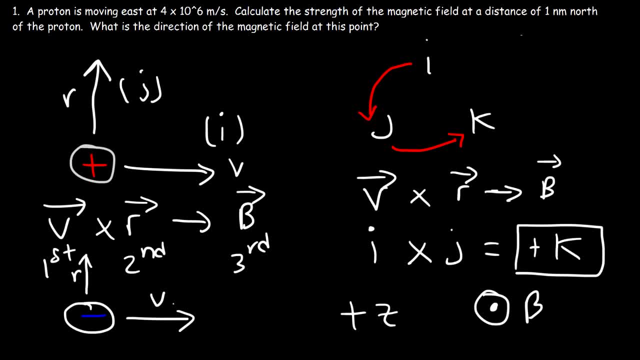 And let's say the position vector is the same and the velocity vector is the same. What is the direction of the magnetic field? The direction of the magnetic field for an electron is simply opposite to that of a proton. So you need to follow everything that you've done so far. 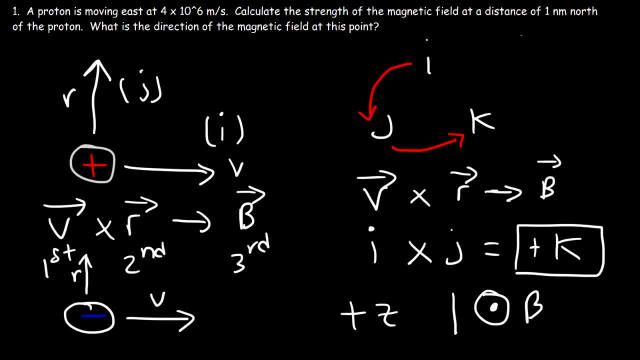 and then just flip your answer. So for a proton, it's going out of the page in a positive Z direction, So we're going to use a circle to represent that, And then just flip your answer. So for an electron, it's going to be going into the page that is in a negative Z direction, with 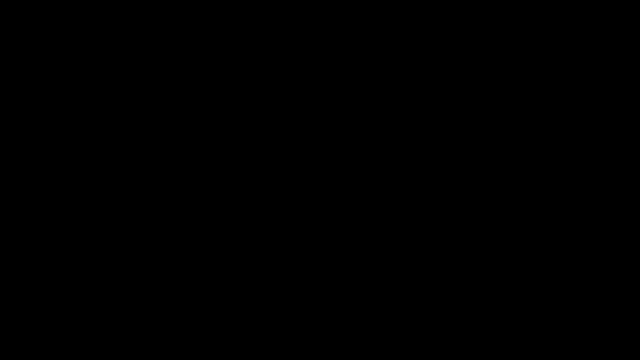 everything else being the same. So let's work on some more examples. Let's say if we have a proton, and this time the velocity is in the Y direction, and we wish to calculate, let's say, the magnetic field at point A, So to draw the position vector. 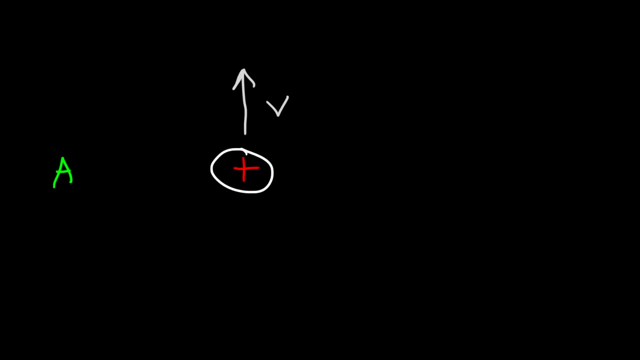 it's going to be from the source vector to the negative Z direction. So we're going to use a circle to represent the force point, which is where the positive charge is located, towards the field point where we wish to determine the magnetic field. So the position vector goes from the charge to the 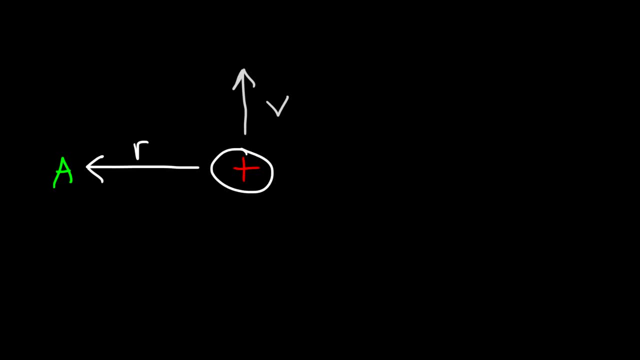 location where we wish to calculate the magnetic field. So let's determine V, cross, R, the sign that this leads to. So first let's use the right-hand vector. So the first vector is going to be associated with the thumb And that's where the velocity is going. 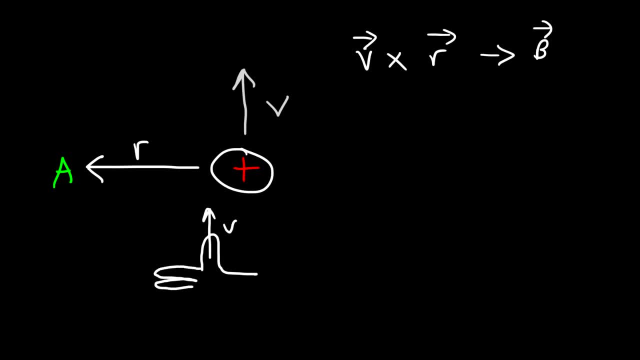 The second vector is associated with the four fingers, And so the position vector- that's the second one- it's going west And the force is once again coming out of the page. So, because I mean not the force but the 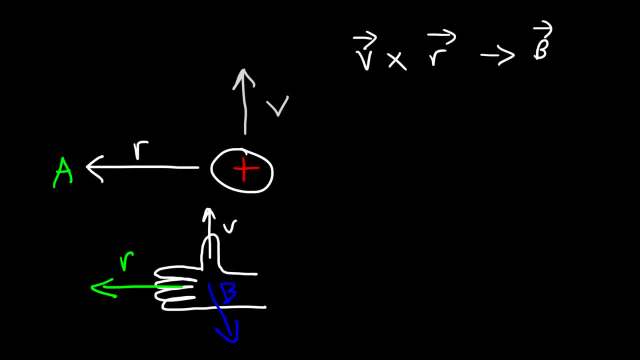 magnetic field is coming out of the page, And so we're going to use a circle to represent that. So it's in a positive Z direction, which is associated with positive K. Now let's use that IJK technique to get the same answer. 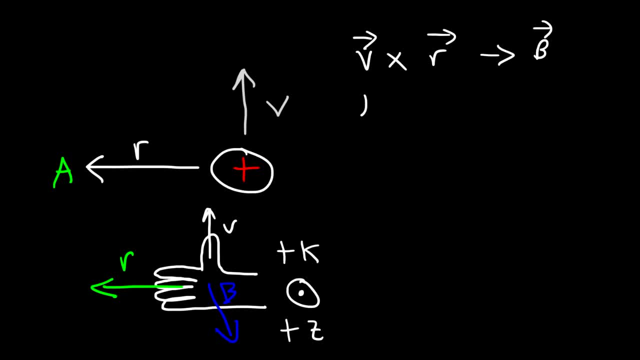 So the velocity is in the positive Y direction, So that's positive J And the position vector is in a negative X direction, So that's negative I. And let's see what that's equal to. So first let's find out what J times. 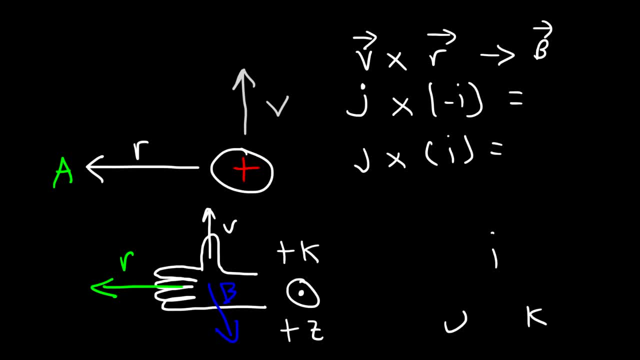 or the cross point product of j and positive i is. So, starting with j, the first vector, we're going to go towards i and that's going to lead us to k. Now, is this equal to positive k or negative k? 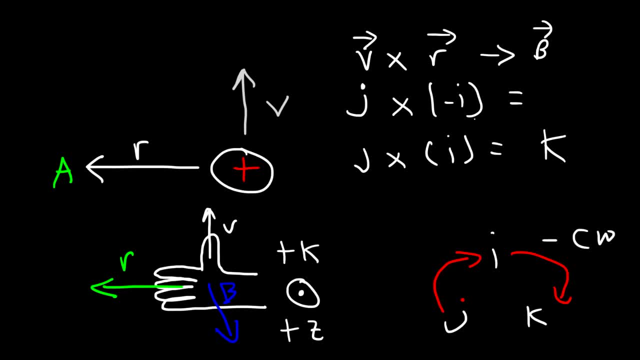 Because we're moving clockwise, we're going to get a negative answer, and this works if all of these are initially positive first. So the cross product of positive j and positive i, according to this diagram, is negative k, since we're going clockwise. 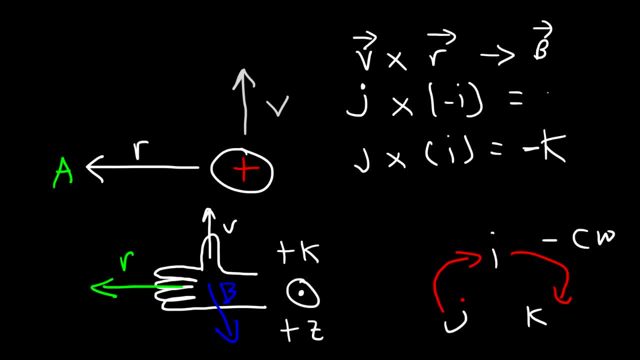 So if we introduce a negative sign here, then this has to change to positive k. If the cross product of j and i is negative k, the cross product of j and negative i is positive k, And this answer is in agreement with what we have here. 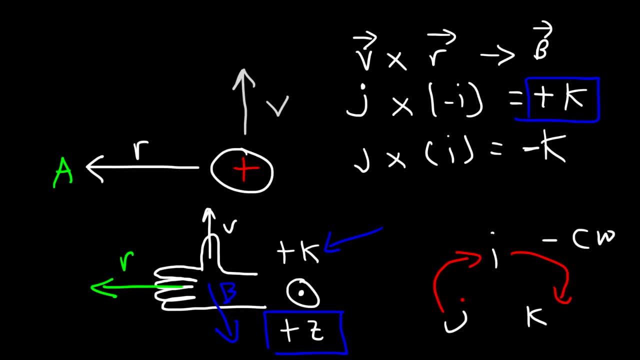 So the magnetic field is coming out of the page into or along the positive z axis, And so you have two techniques in which you could determine the direction of the magnetic field, and you know how to calculate them, The magnitude of the magnetic field, which we did in the beginning of this video. 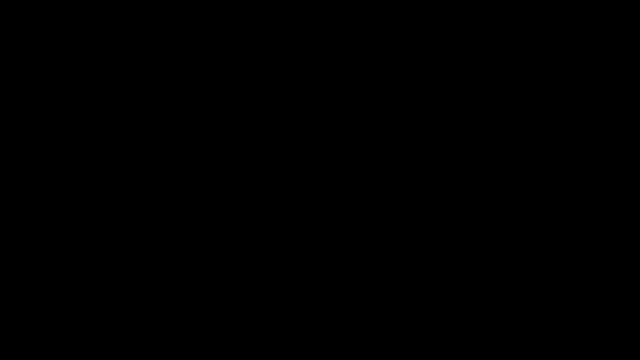 Now let's say if the proton is moving out of the page, So the velocity is in a positive z direction. So that's going to be represented with positive k. And let's say we wish to calculate the magnetic field at this point, So the velocity is in a positive z direction. 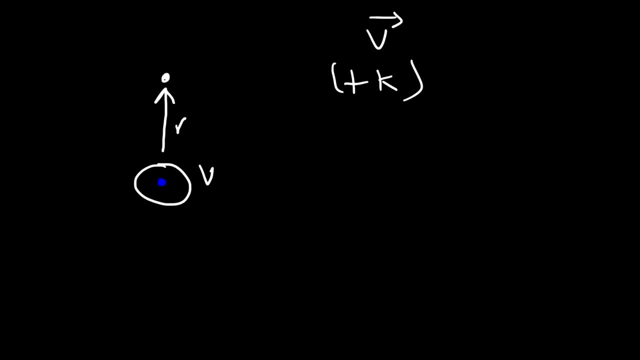 The position vector goes from the charge to the point of interest. What is the direction of the magnetic field in this case? So the position vector is in a positive j direction. So, using the right-hand rule, your thumb has to be pointing out of the page. 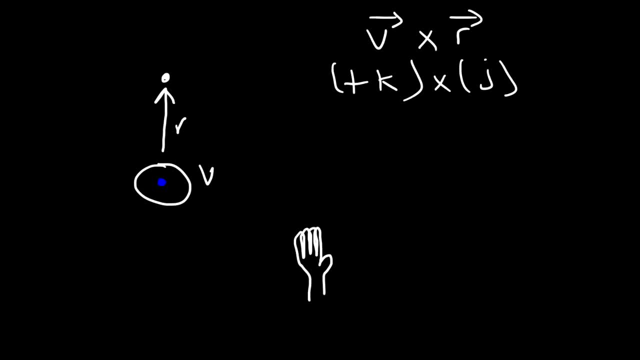 and your forefingers have to be pointing north, So your forefingers are going this direction and your thumb is going out of the page, And so the magnetic field which comes out of the palm of your hand is directed towards the left. 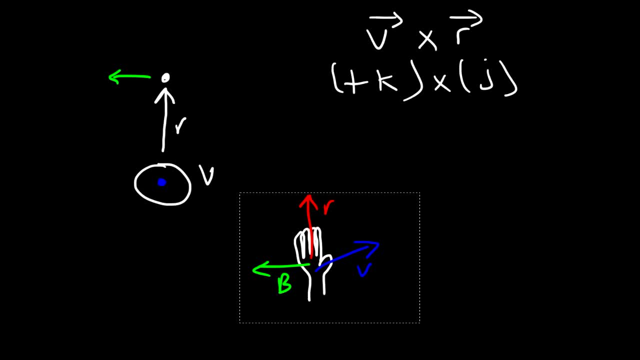 So it's going in this direction. So, using this technique, we're trying to figure out k times i. I mean not times i, but k times j. So we're going in the clockwise direction, And so that's equal to negative i. 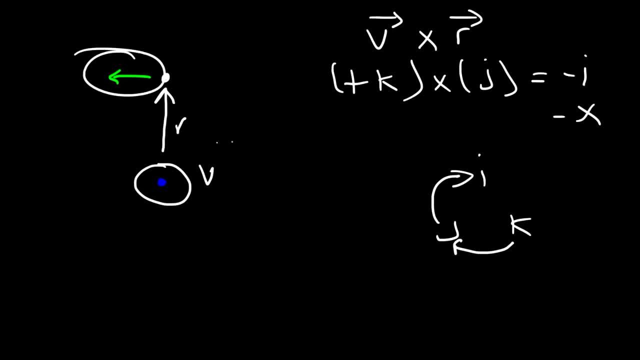 And negative i is the same as negative x, which this is going west. So that works. So now, what about at this position? What is the direction of the magnetic field at that position? So let's find out, Let's find the cross product of these two vectors. 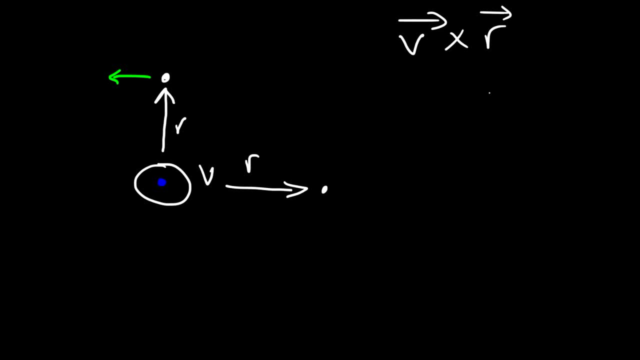 So once again, the velocity is in the positive z direction, So that's k, And the position vector is now in the positive x direction, So that's i. So we've got to find the cross product of k and i. So we're going to start with k first and then go towards i. 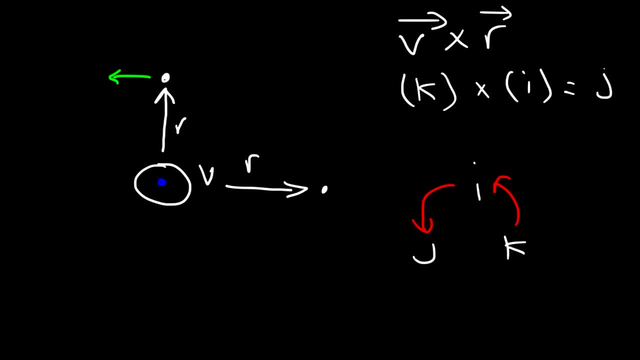 And this is going to lead us to j, And because we're going counterclockwise, this time this is positive j, Which means that it should be going in the positive y direction, So the magnetic field is going in the positive y direction. 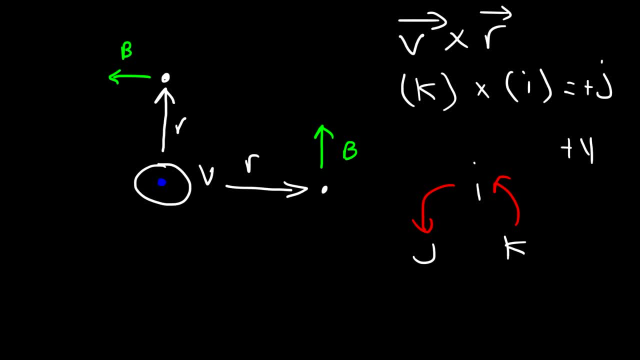 And it's going in that direction. So now, if we wanted to find it at this point, we could just complete the circle, So we can see that the magnetic field is circular. It's actually counterclockwise if the proton is moving out of the page. 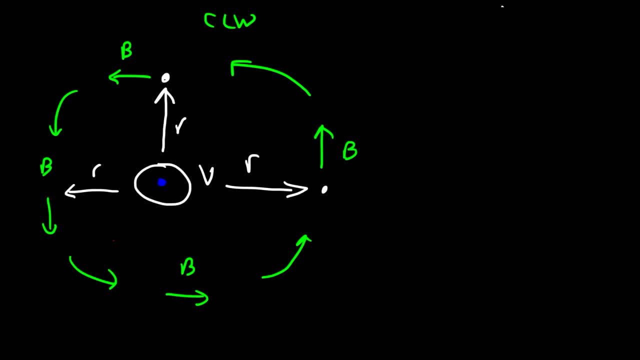 So the reverse must be true as well. If the proton is moving into the page, then the magnetic field is going to be clockwise around the proton. For an electron you simply have to change the direction. So let's say, if this is the proton,